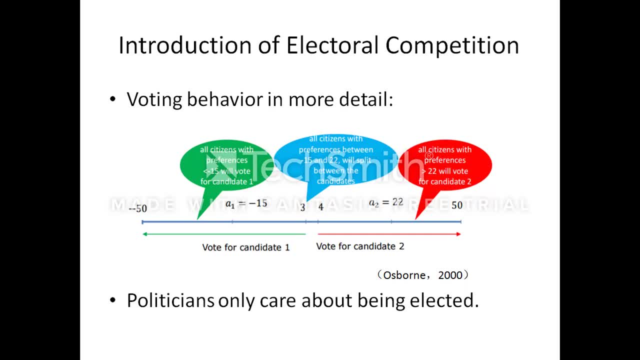 minus 15 will, of course, vote for candidate candidate 1, since they closer to player 1 than player 2.. In the same logic, all citizens with preferences larger than 22 will vote for the player 2.. All citizens between minus 15 and 22: 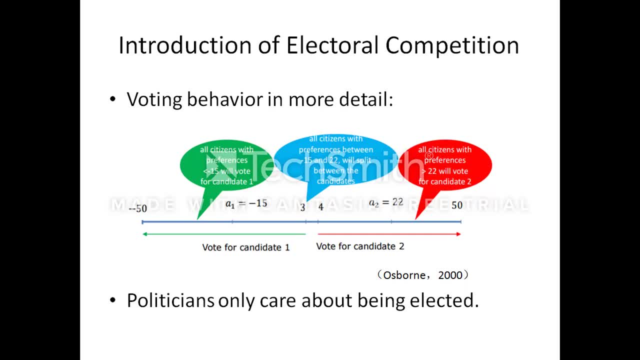 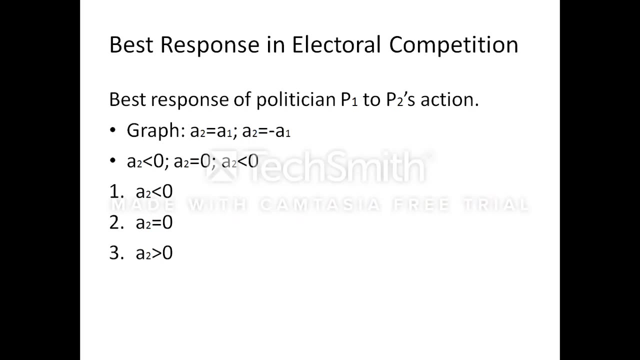 will split between the candidate. It is worth to mention that the politicians only care about being elected, so they only care how to get more vote. Based on this assumption, let's come to the second part: best response in Electro competition. Let's see the best response of politician 1,. 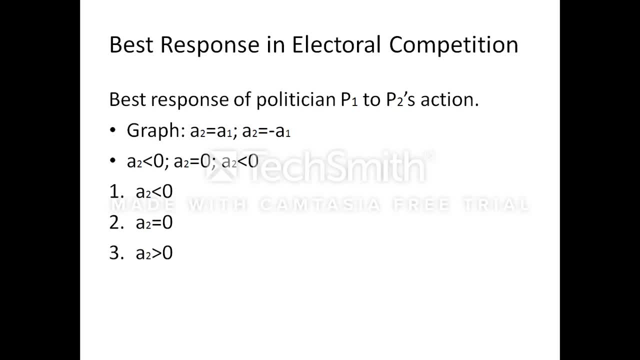 politician 2's action first. We will get the best response function by drawing graphs, since we have the choice from minus 50 to 50, which is involving both positive number and negative number. So in the graph we must have two lines which are A2 the same with A1 and A2 is the same. 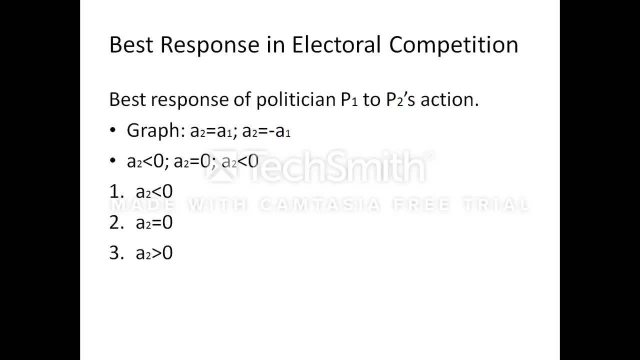 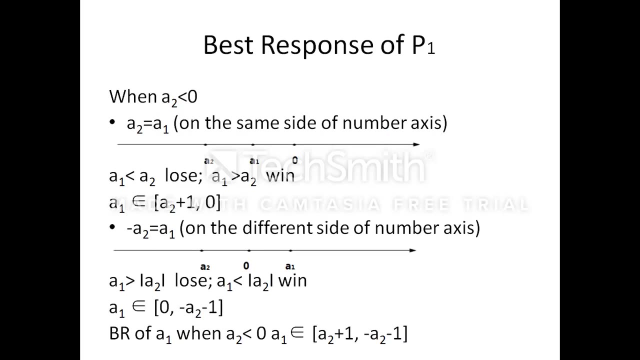 with minus A1.. The action of partition 2 has three situations. The first is A2 smaller than 0, the second is A2 is the same with 0, and the third one is A2 is larger than 0.. When the choice of player 2 is smaller than 0, as mentioned before, we have two classifications. 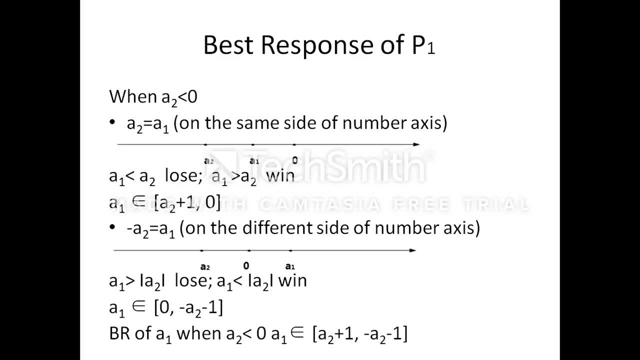 A2 is the same with A1 and minus A2 is the same with A1.. When A2 is the same with A1, this implies that both players in the same side of the number axis. We can see the graph here. It is quite obvious that if A1 is smaller than A2, player 1 will. 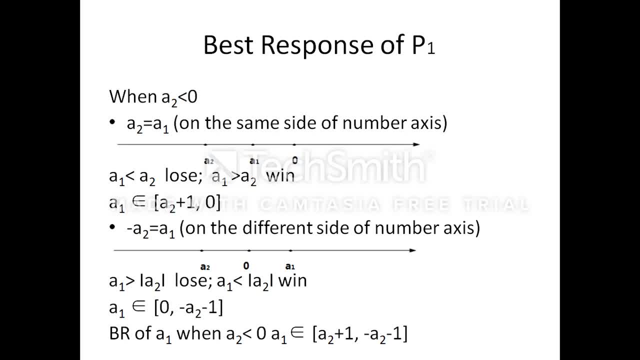 lose, while player 1 will win if A1 is larger than A2.. So the best response of player 1 is choosing the action belonging to A2 plus 1 and 0. When minus A2 is the same with A1, this implies that the action of players are in the different. 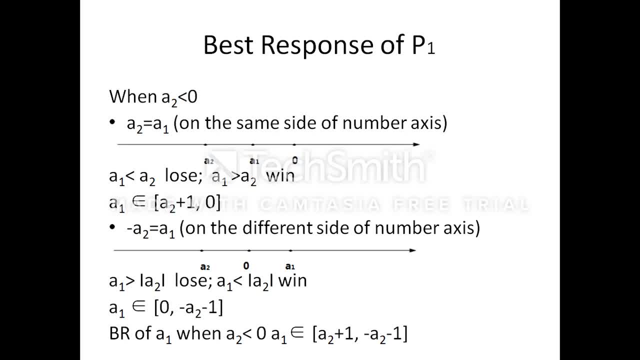 side of the number axis, As shown in the slide, we can easily find out: player 1 will lose when A1 is larger than absolute value of A2, while player 1 will win when A1 is smaller than absolute value of A2.. Based on these two situations, we can conclude that the best response function of 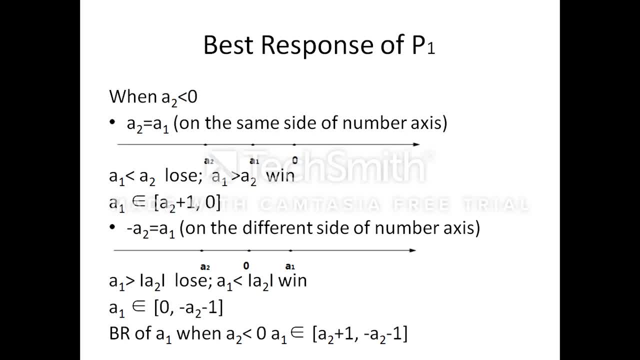 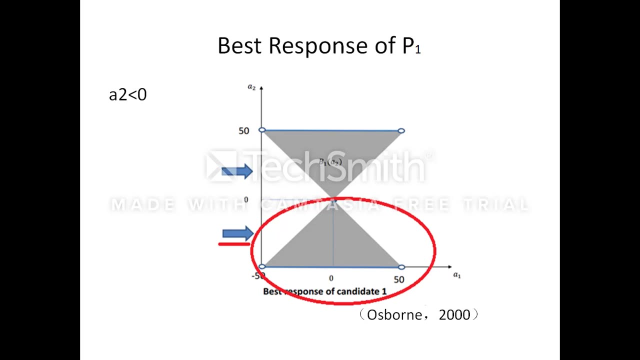 player 1 when A2 is smaller than 0, is A2 belong to the interval from A2 plus 1 to A2 plus 1 and 2 minus A2 minus 1.. The graph of best response of player 1 is showed, labeled by red circle, when A2 is smaller than. 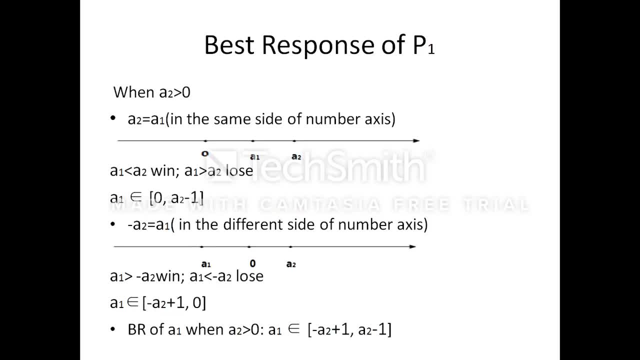 0. Now let's come to the second situation, When the choice of player 2 is larger than 0, the same logic as what we mentioned in A2- smaller than 0. We have two options here. We have two classifications: A2 is the same with A1 and minus A2 is the same with A1. When A2 is the 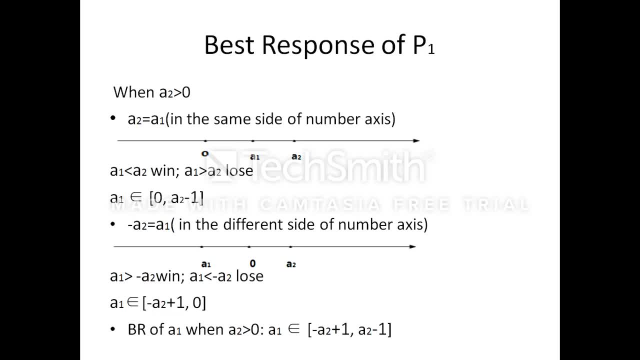 same with A1, player 1 will win when A1 is belong to the interval of 0 and A2 minus 1.. When minus A2 is the same with A1, the best response of player 1 is belong to the interval. 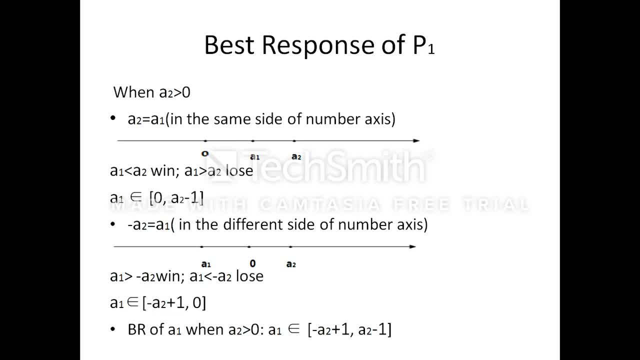 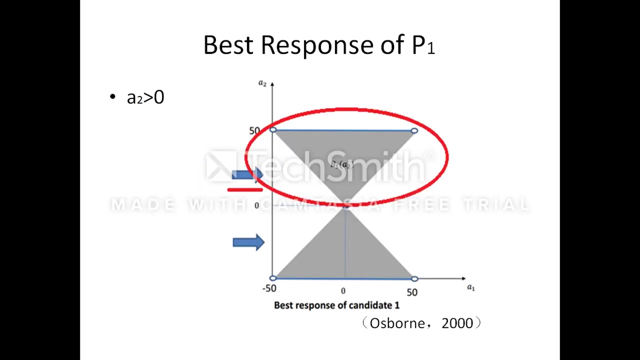 of minus A2, plus 1 and 0.. Combine these two situations together and we could know that the best response of player 1 when A2 is larger than 0 is A1 belong to the interval of minus, A2 plus 1 and A2 minus 1.. Here is a graph shows the best response of player 1, which 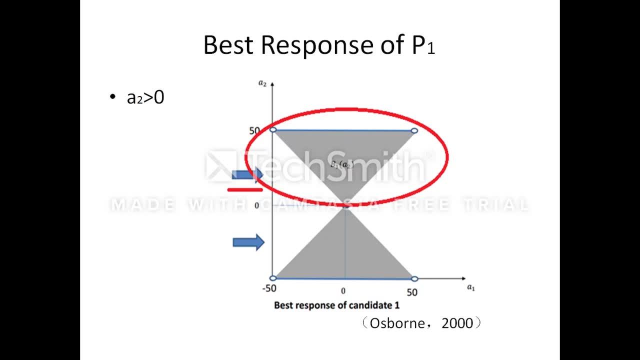 is labeled as red circle when A2 is larger than 0.. Now let's come to situation when A2 is the same with A1.. Now let's come to situation when A2 is the same with A1 when A2 is larger than 0. When 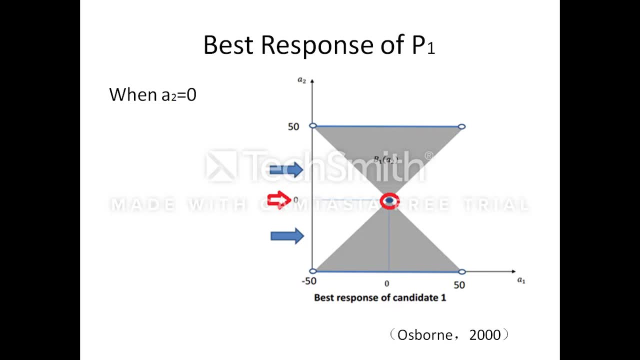 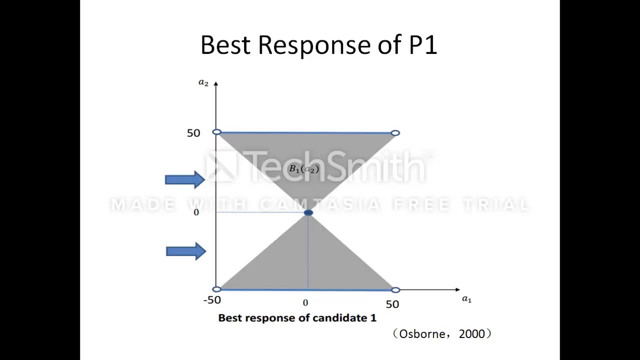 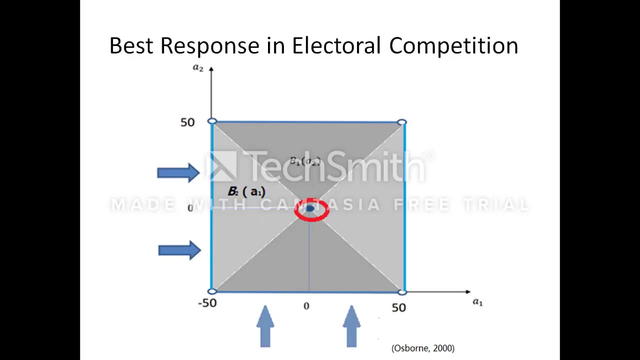 The best response of player 1,, of course, will be 0 if player 1 doesn't want to lose. So here is a complete version of best response of player 1.. And the best response of player 2 is symmetric with player 1..